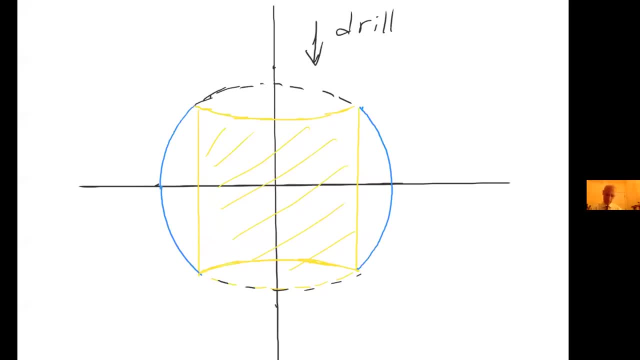 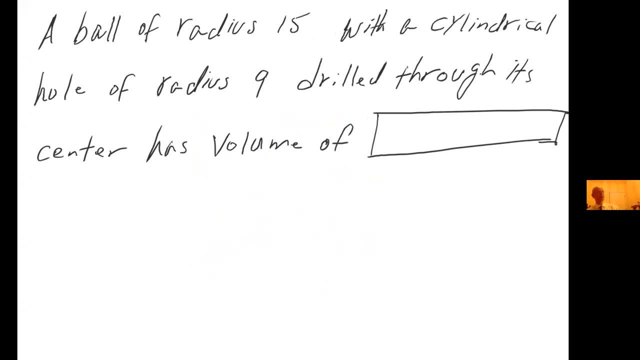 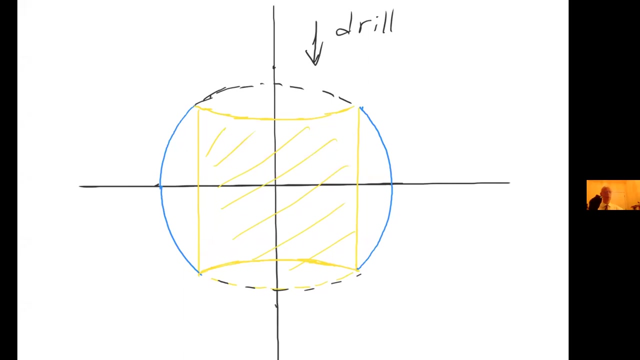 We have a bald spherical ball of radius 15 with a cylindrical hole of radius 9.. Drill through it. It's centered. It has volume off. So our job is to find the volume of. let me go to the next page. Here it is, So we do have just pretend that the circle is sphere. 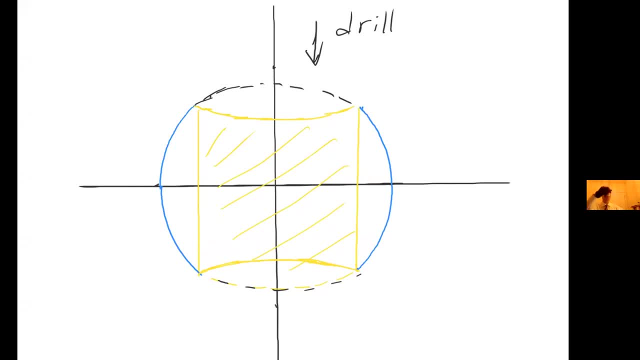 a three-dimensional sphere and we drill a hole through it. We were told that the sphere itself has so radius 4, radius of sphere e cones, according to this problem, 15, and radius of the cylinder that we drilled is 9.. And we are trying to find the volume. 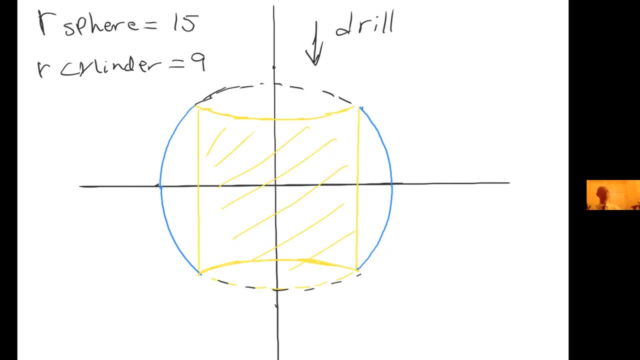 of the, whatever, that is, the drilled sphere. So notice that, first of all, if I put the center of this sphere at 0, 0, and say this is x, this is y, two things I can do. First of all, I can claim that x to the. 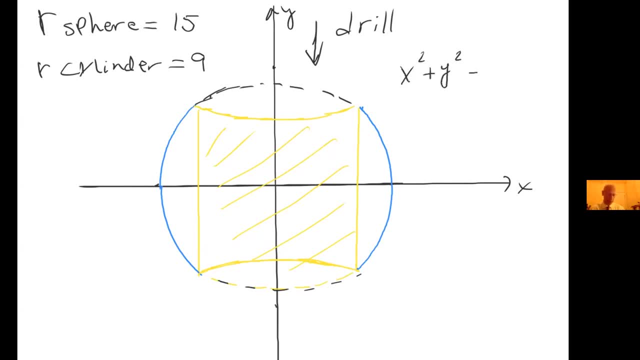 second plus y to the second equals 15, squared is 225.. I can also claim that y squared equals 225 minus x squared and y equals a square root of 225 minus x to the second, And here is 0, 0.. And notice that if I find the volume 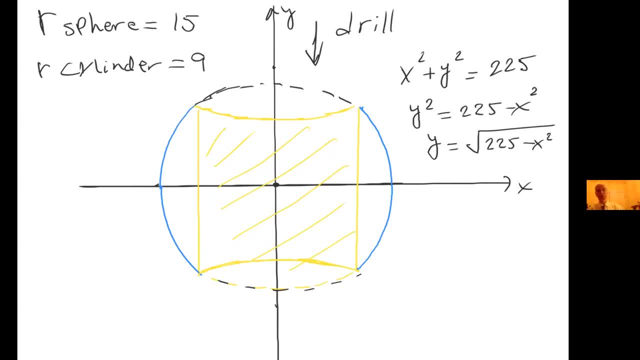 of the upper half. it's the same volume as the lower half. So that's what I'm going to do And I'm going to go ahead and take advantage of that. So every cylinder in here, every cylinder that I go, so let's say, let me choose. yeah, this is. 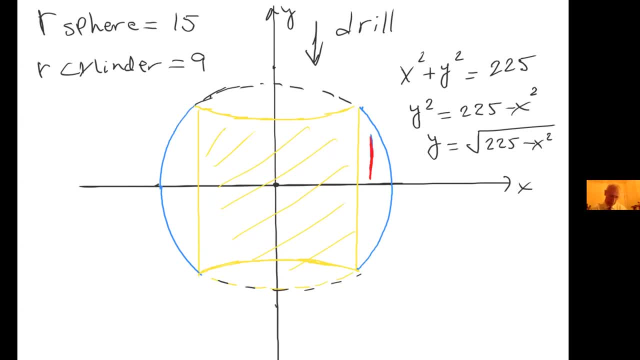 I'm going to go by it. So let's say, if I have one cylinder, that is goes here. Okay, What is the radius? The radius of my cylinder equals simply x. What is the height of the cylinder? Height of the cylinder is square root of 225 minus x squared. 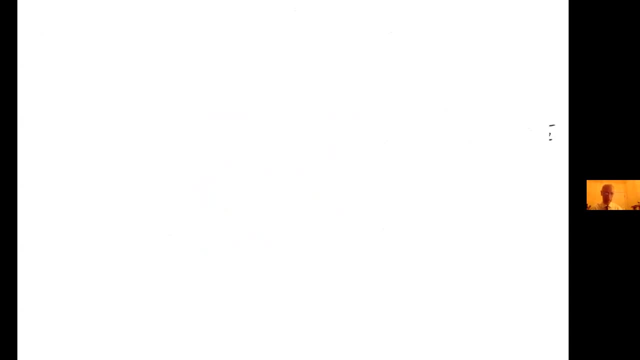 So let me go go ahead and go to the next page, And so here's what I'm going to do. First of all, I'm going to remember that I'm using symmetry, So I'm going to say two. this two is because 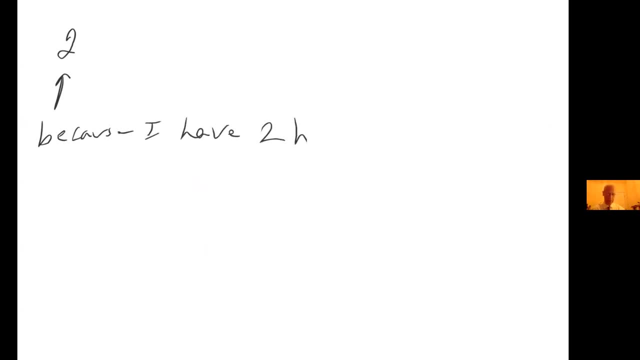 I have two halves Half sphere, Okay, And if I take the integral from 9 to 15, the radius of every cylinder is 2 pi r, in this case, 2 pi radius And times the height, the height or. 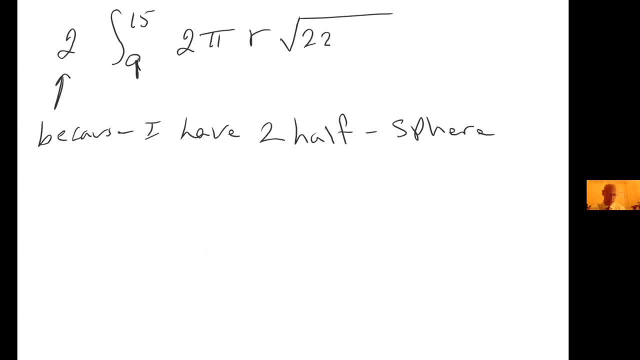 y value is square root of 225 minus x, squared All this dx. So if I pull the 2 pi out I'm going to get 4 pi from 9 to 15.. And we said that the radius actually is x, and so 2 pi x. 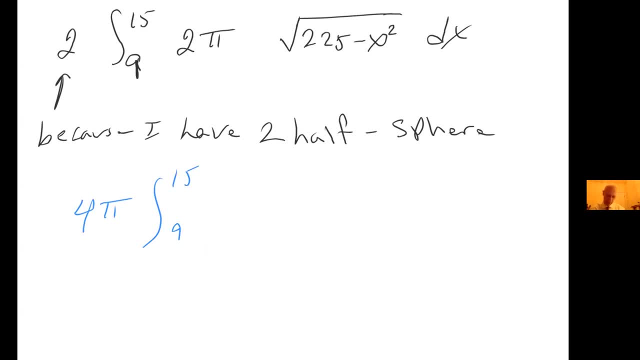 x, 2 pi x x score root of. well, actually I took my two pi out, So two pi x times score root of 225 minus x squared dx. Let me double check my work. Let's see, First of all, the boundaries of integration. 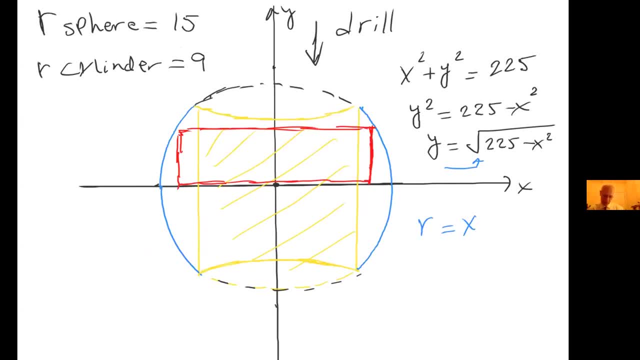 So we said that this, the radius of the drill, is nine, So I want to go from nine to 15, that's correct. The radius, let's say the radius of this red, this red cylinder right here is the r- is simply x.